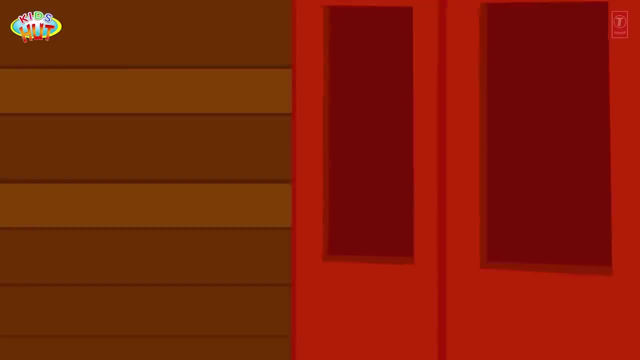 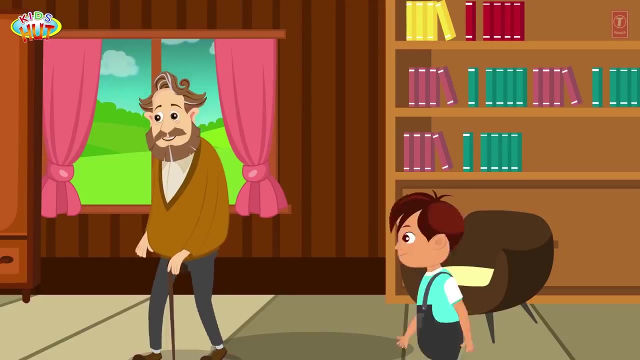 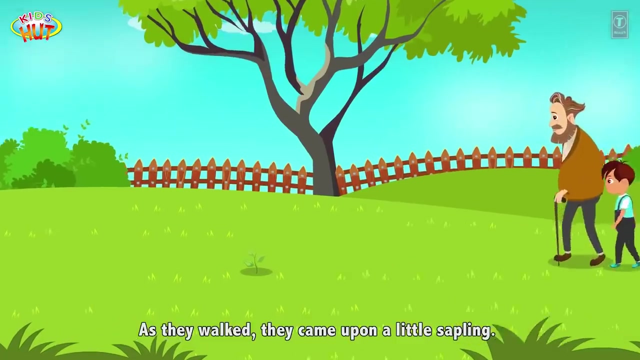 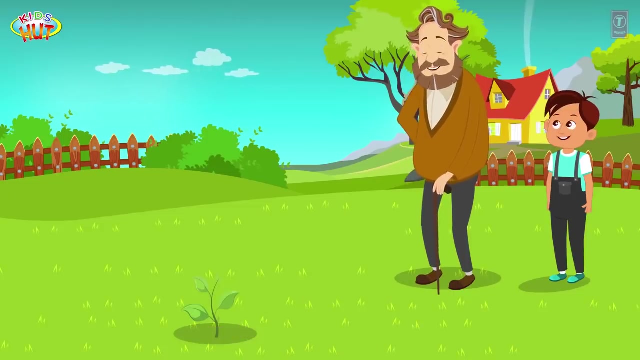 He brought his boy to him. Come, son, let's go for a walk. The boy obeyed and they went for a walk in the garden. As they walked, they came upon a little sapling. Son, pull out the sapling for me. 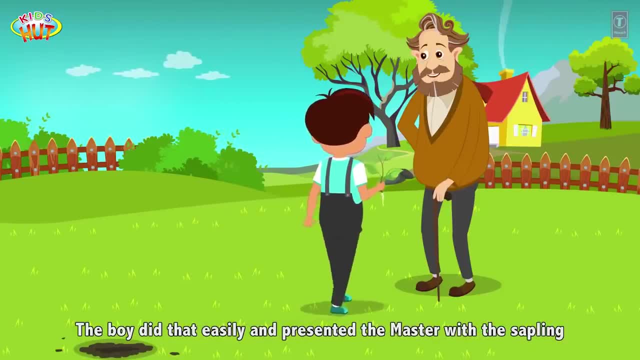 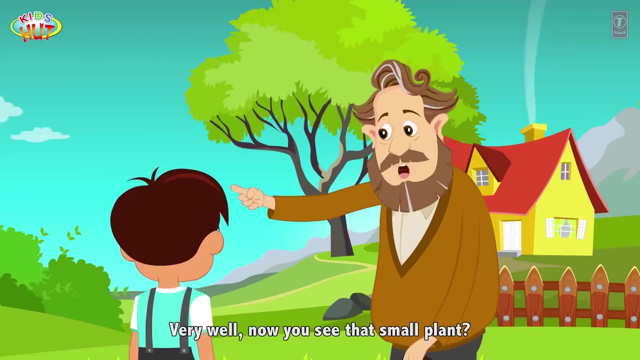 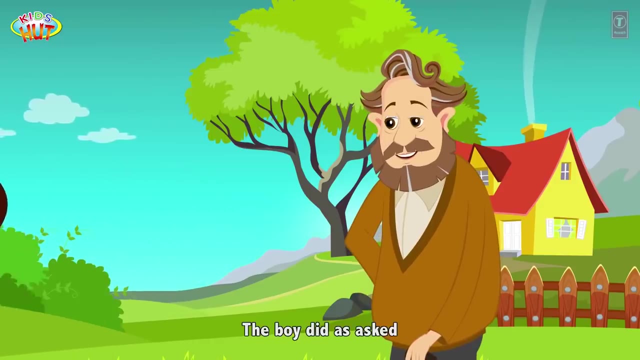 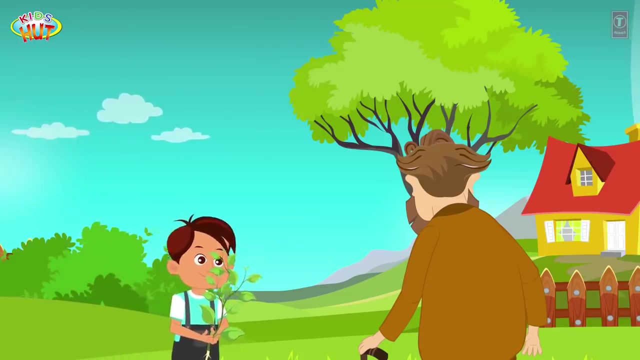 The boy did that easily and presented the master with the sapling. Very well, Now you see that small plant, Pull that out for me. The boy did as asked and easily pulled the plant out. Next, the master asked him to pull out a bush. 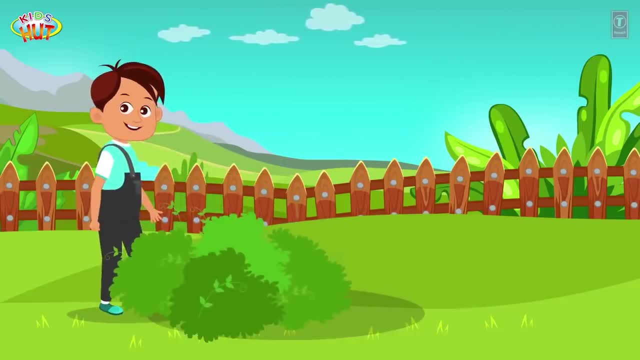 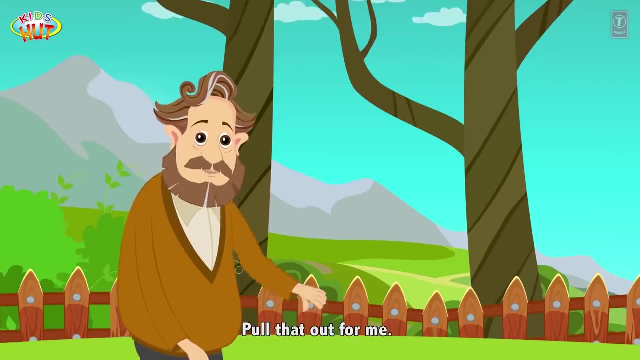 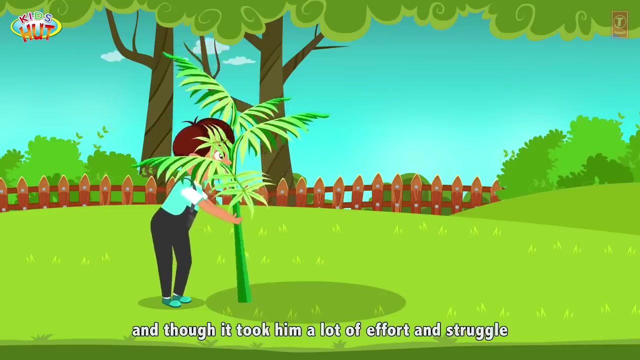 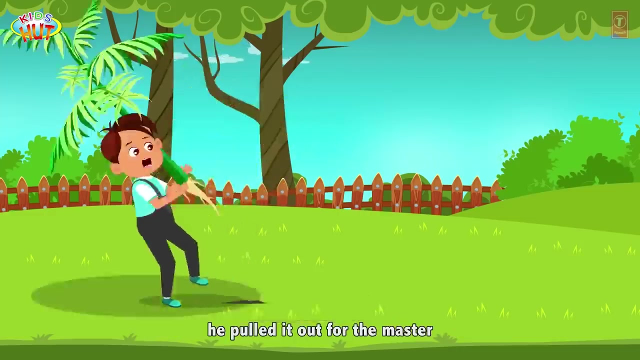 It took some effort, but the boy did that too. Now see that small tree, son, Pull that out for me. The boy went to the small tree and though it took him a lot of effort and struggle, he pulled it out for the master. 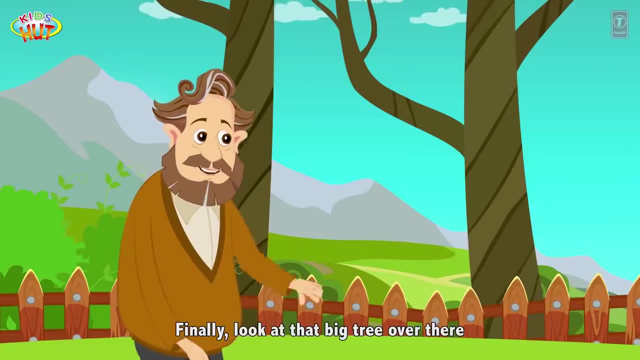 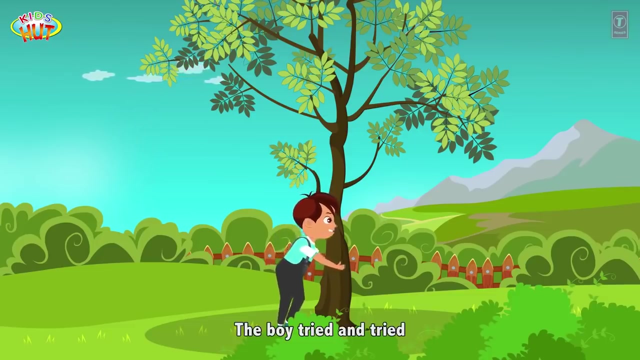 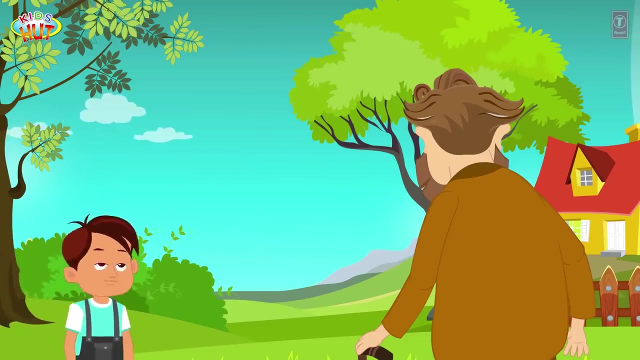 Very well done. Finally, look at that big tree over there. Pull that out too for me. The boy tried and tried, but the tree did not budge. Finally, tired, the boy gave up. I am sorry, wise master, I cannot pull that tree out. 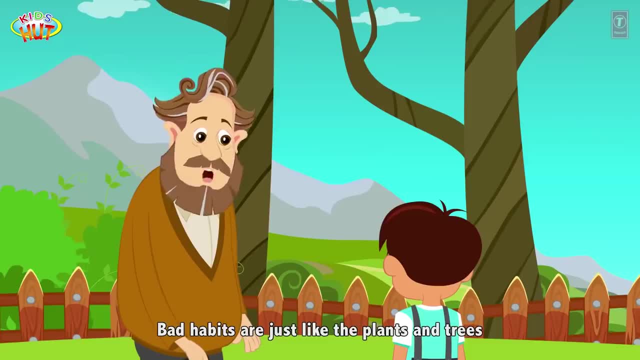 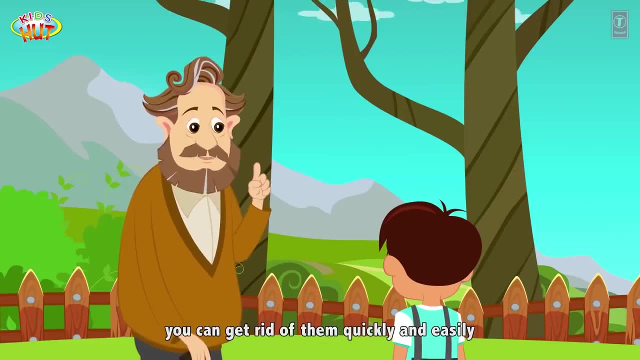 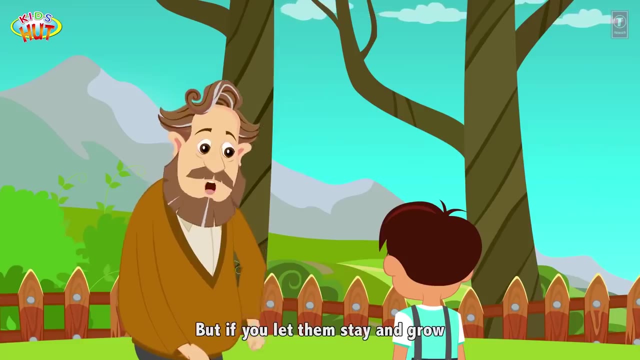 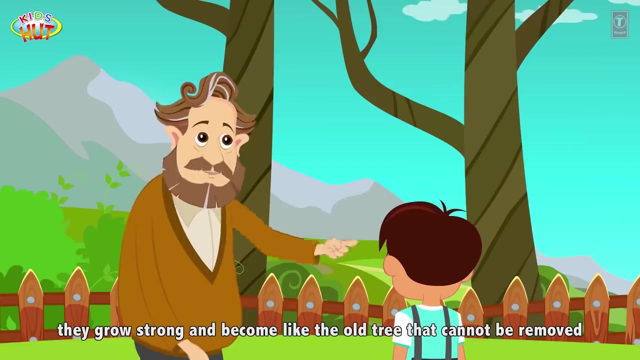 It is old and strong. Bad habits are just like the plants and trees. When they are new, like the sapling, you can get rid of them quickly and easily. But if you let them stay and grow, they grow strong and become like the old tree that cannot be removed. 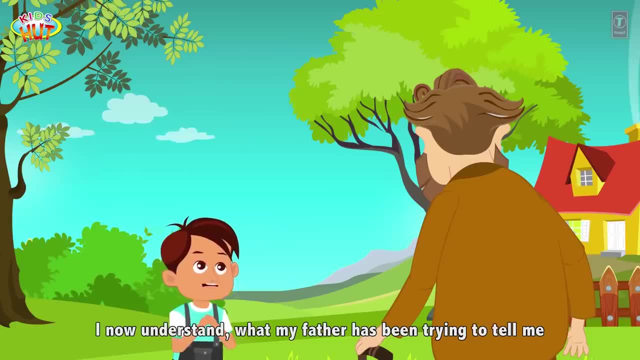 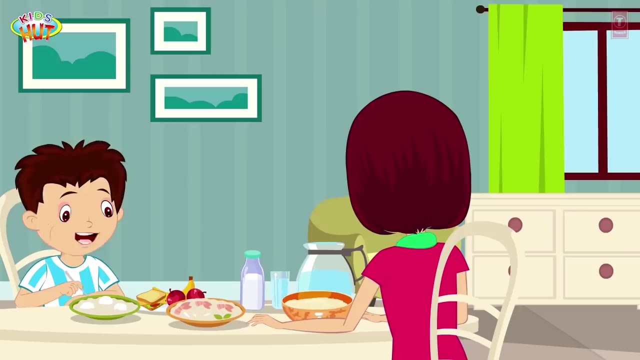 Forgive me, master. I now understand what my father has been trying to tell me. I will drop all my bad habits from now on, Dear. what if talking with food in my mouth becomes my bad habit too? I will stop it right now. 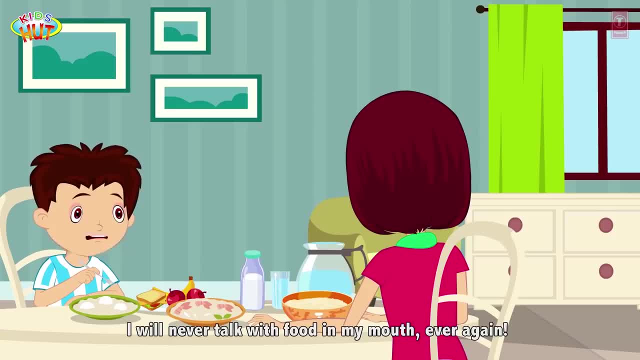 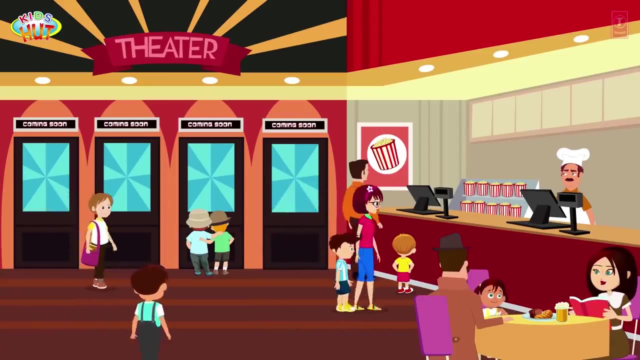 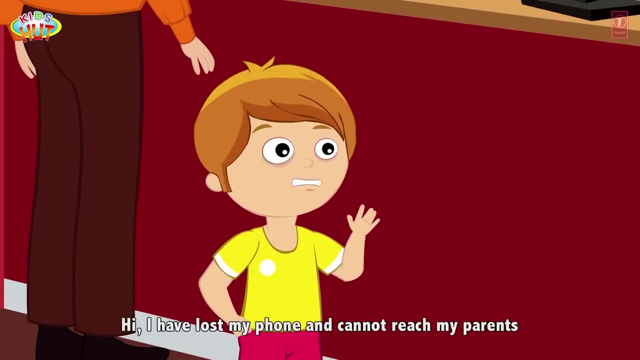 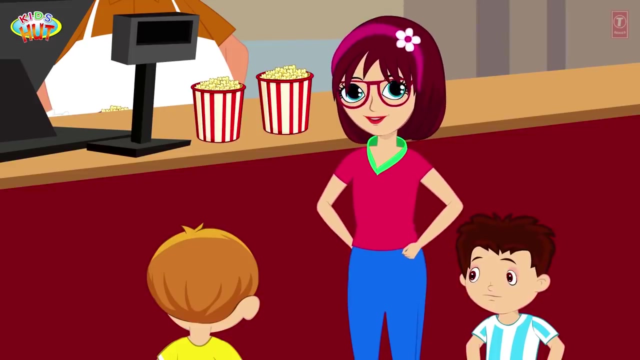 I will never talk with food in my mouth, ever again. That's great. Thank you, Tofu. Hi, I have lost my phone and cannot reach my parents. Can you please help me make a call home? Yes, sure I can take you to the theatre manager. 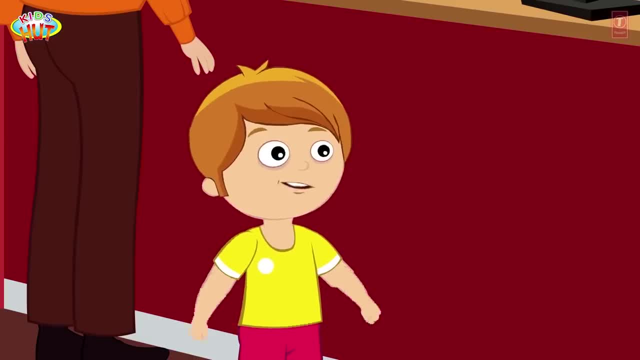 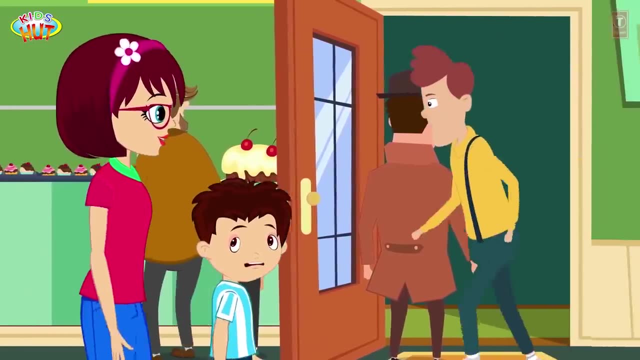 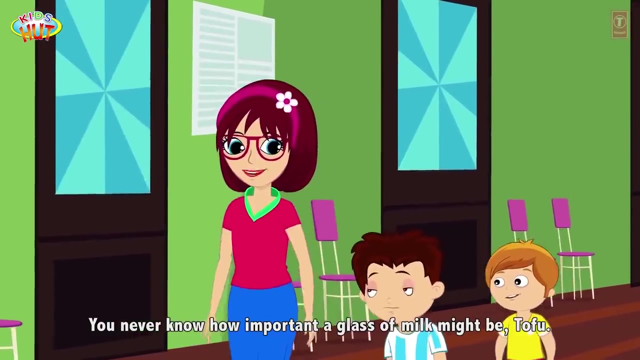 He will have a phone. Thank you, Tia. what are you doing? We will miss the start of the movie. We don't even know this boy. You never know how important a glass of milk might be. Tofu, What? 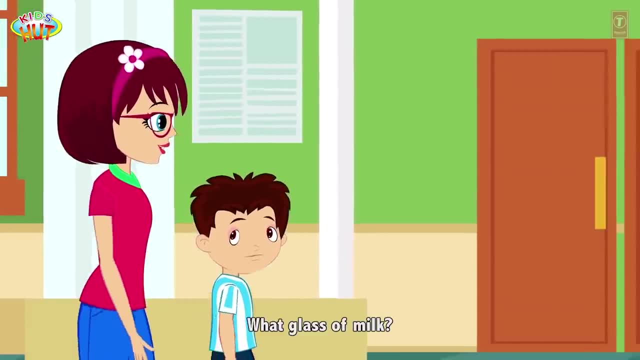 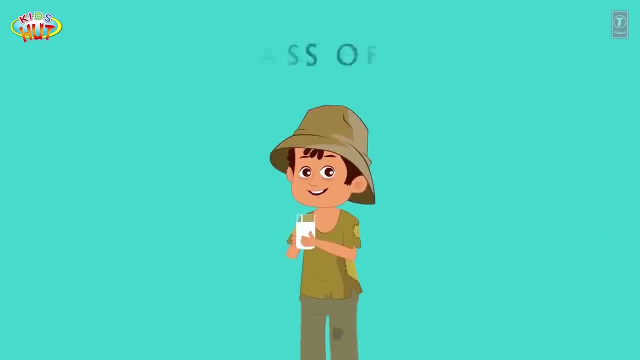 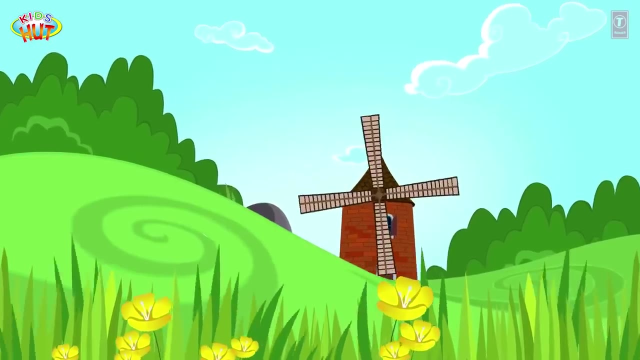 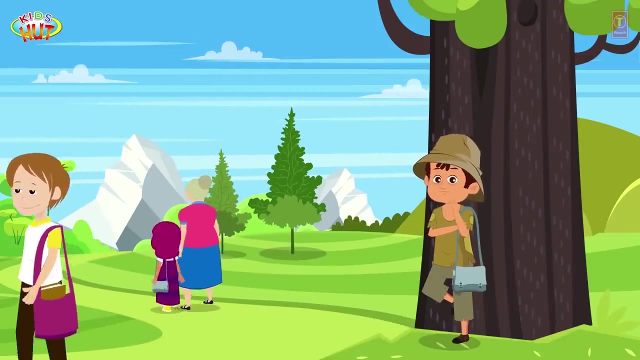 What are you talking about, Tia, Tia, what glass of milk? You'll know in a minute. Glass of Milk. Once upon a time there lived a young boy who was very poor. He did odd jobs to be able to buy his daily food and go to school. 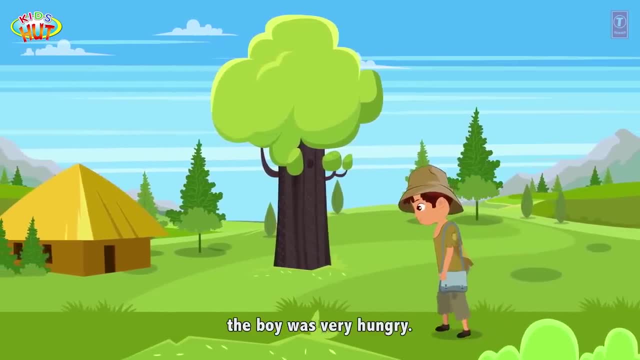 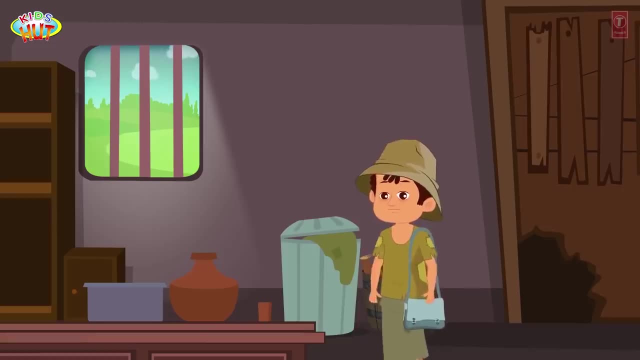 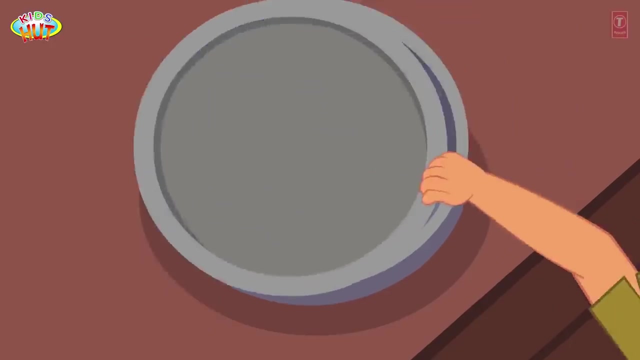 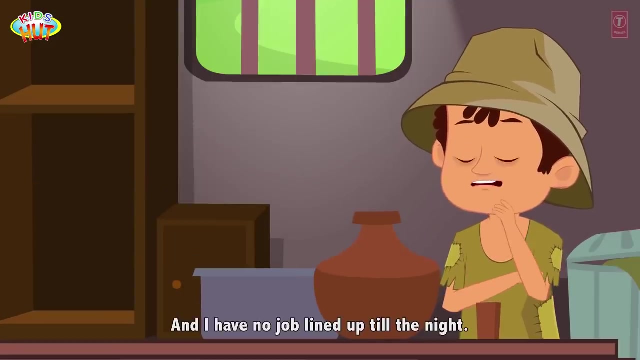 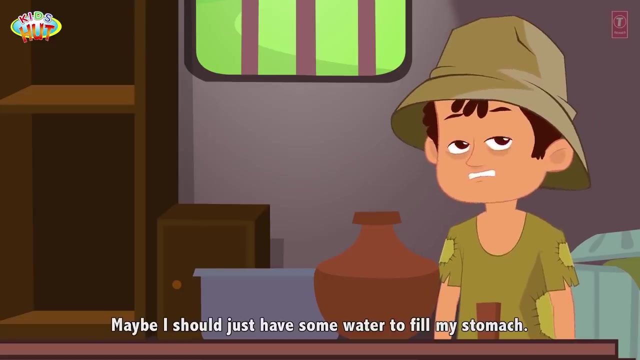 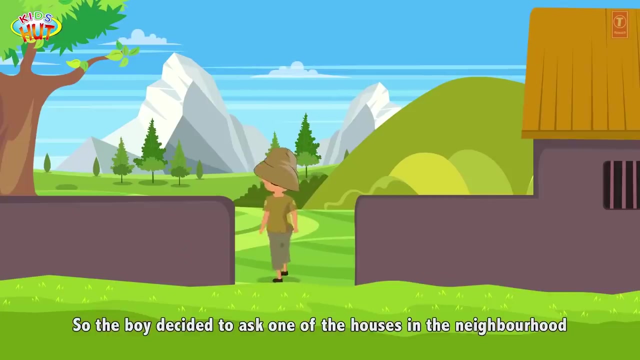 One day after school, the boy was very hungry. I don't have money today and I have no job lined up till the night. How will I make it through the day? Maybe I should just have some water to fill my stomach. So the boy decided to ask one of the houses in the neighbourhood for a glass of water. 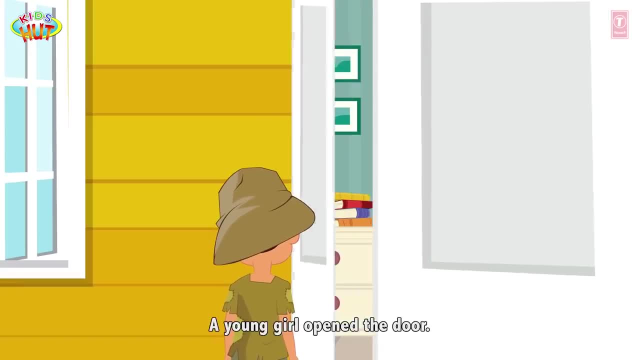 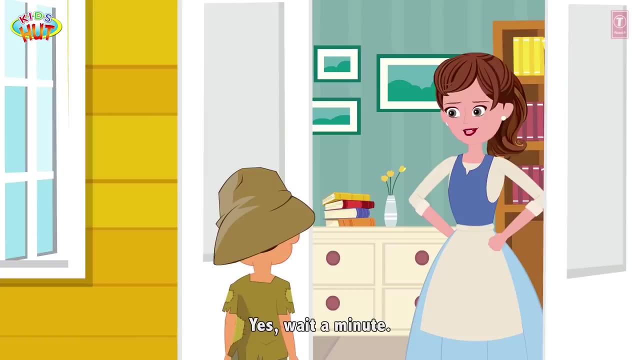 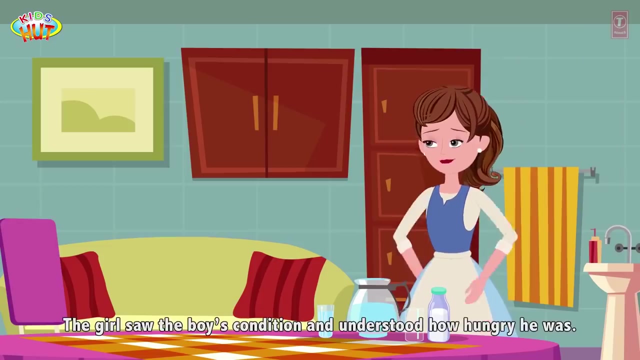 He knocked on the first door, A young girl opened the door. I am very thirsty. Can you please give me a glass of water? Yes, Wait a minute. The girl saw the boy's condition and understood how hungry he was. Instead of a glass of water, she brought him a glass of milk. 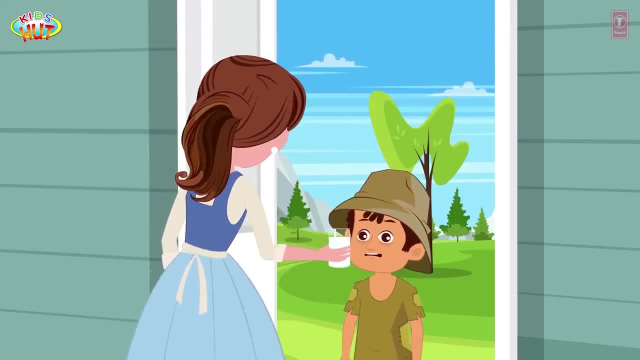 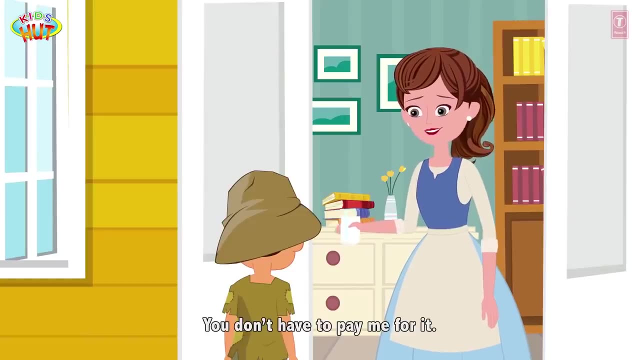 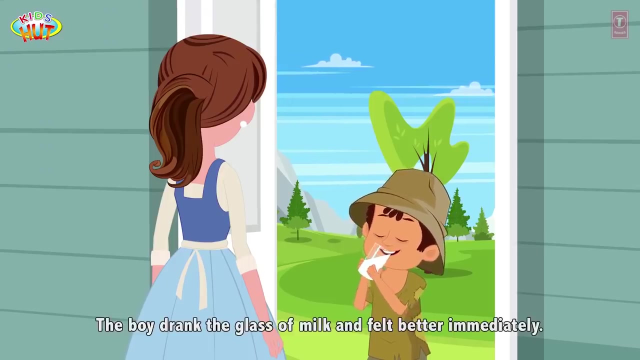 The boy was surprised to see the milk. I cannot take this. I do not have any money to pay you for it. It's okay, You don't have to pay me for it. Oh, Thank you very much. The boy drank the glass of milk and felt better immediately. 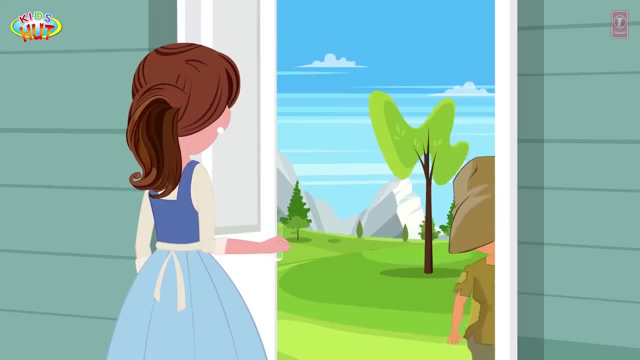 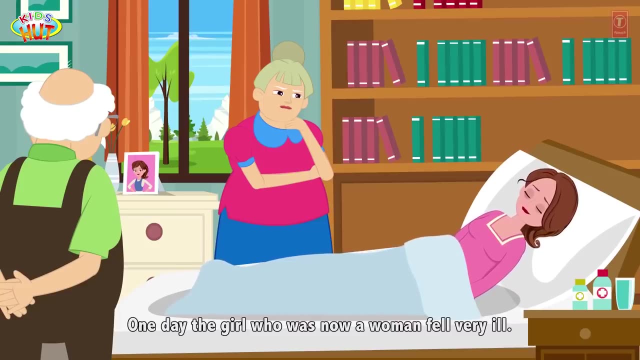 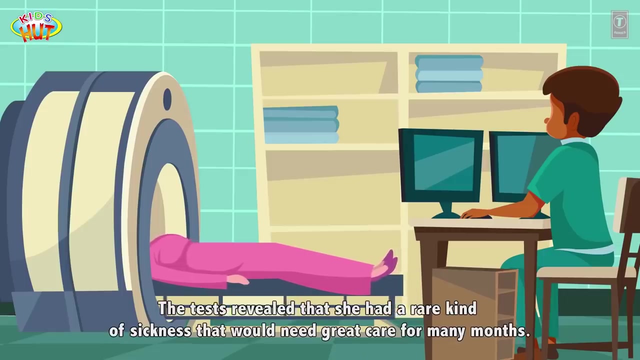 He thanked her and went his way. Many years went by. One day the girl, who was now a woman, fell very ill. She was taken to the hospital. The tests revealed that she had a rare kind of sickness that would need great care for many months. 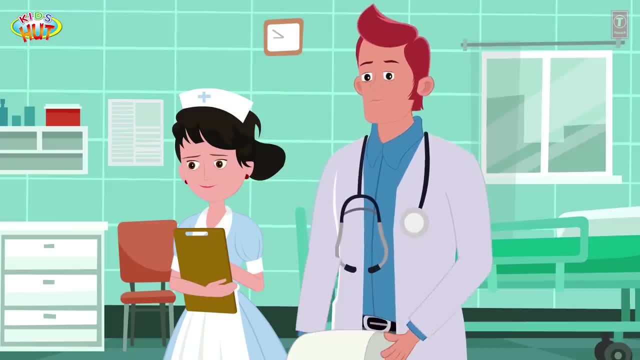 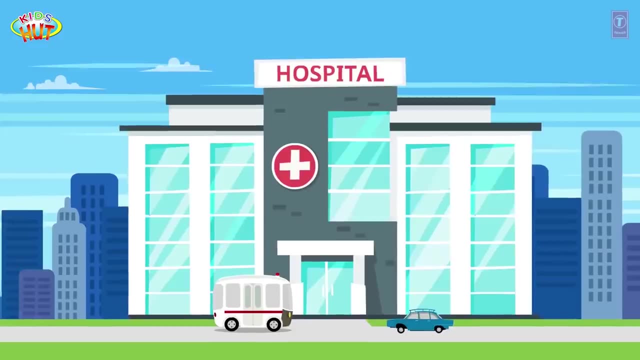 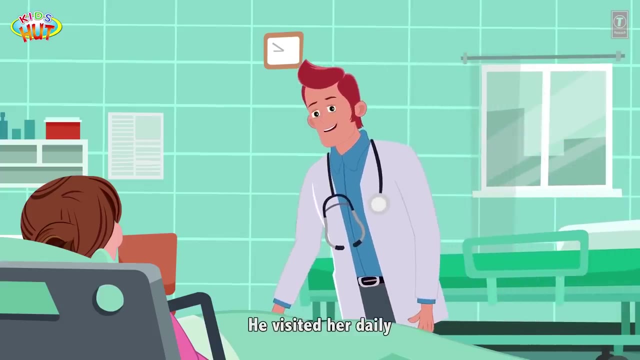 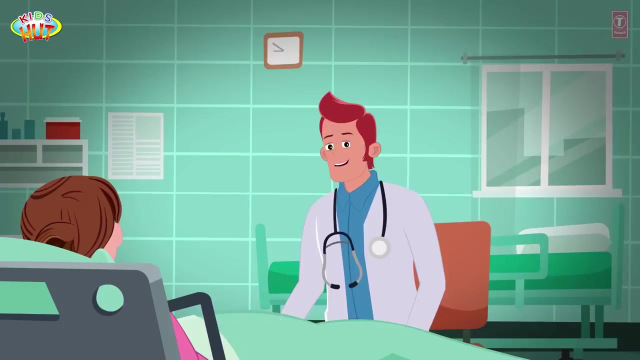 Dr Philip was assigned to her case. Don't worry, We will take care of you. Thank you, As he had promised, Dr Philip took great care of her. He visited her daily, stayed by her bedside at night and made sure she was always comfortable. 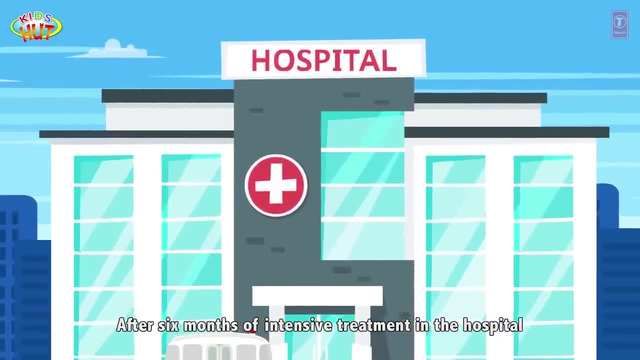 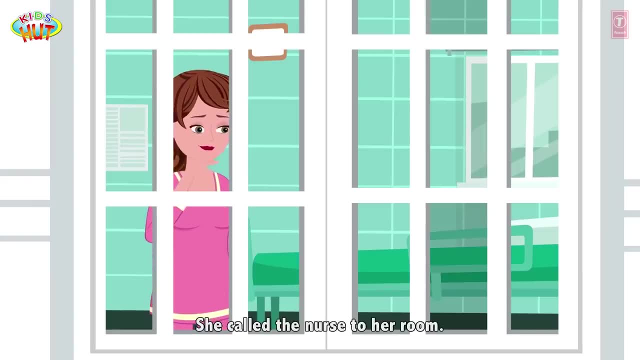 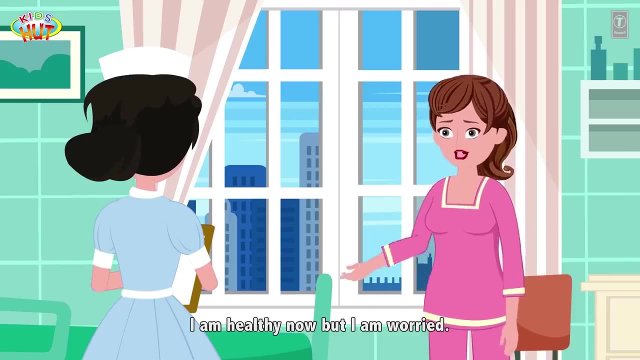 After six months of intensive treatment in the hospital, the girl was finally well and could go home. But she had a worry. She called the nurse to her room. I am healthy now, but I am worried. It is time for me to pay the hospital bill. 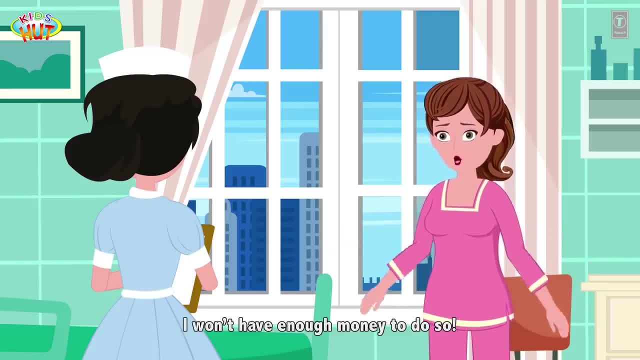 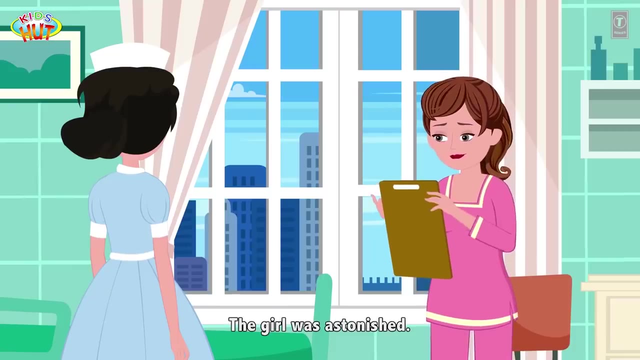 But I am afraid I won't have enough money to do so. Oh, You don't need to worry about it, Your bill has already been paid. What? By whom? Have a look yourself. The girl was astonished. The bill was cancelled across.